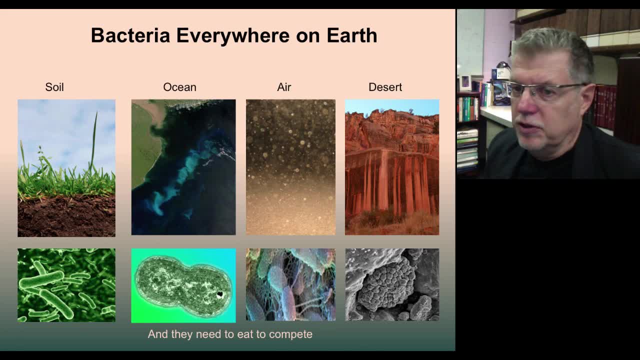 very dry conditions. They can live in the cracks And, in fact, if you look in the desert and you see the color on rocks, often that's due to the pigments of bacteria that are living in the crevices of the rock. The other point is that bacteria are present at enormous quantities. 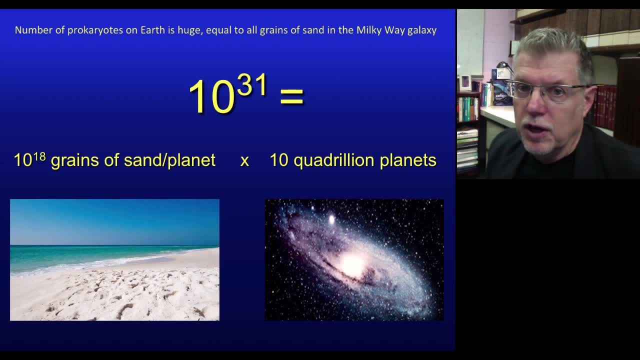 on earth. They are really the most successful living things on earth. So one way to look at this is just sheer numbers. So it's been estimated that there are 10 to the 31 prokaryotes, or 10 to the 31 prokaryotes on earth. Now one way to calibrate thinking about that is say: 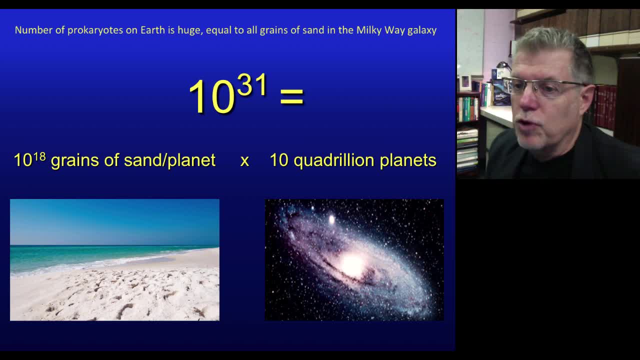 to compare to grains of sand. Well, that's not even close. The number of grains of sand on earth is 10 to the 18.. So let's assume that every planet in the Milky Way galaxy has a planet around it that has sand, like earth. If you took all 10 quadrillion planets. 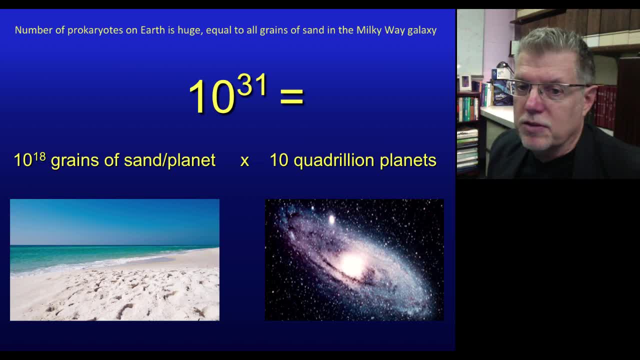 in the Milky Way galaxy. multiplied that by the grains of sand on earth, you'd have 10 to the 31.. So that's what you have to do to get to a number that large, which is the number of bacterial cells on the planet. 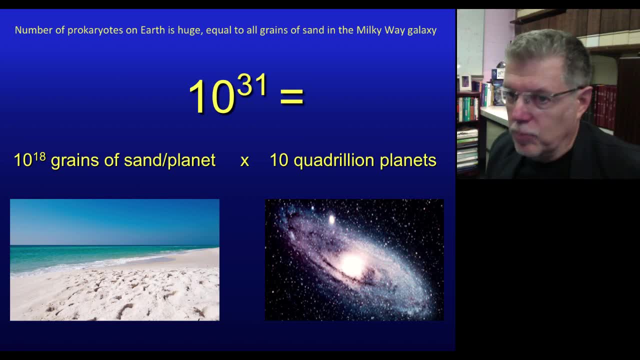 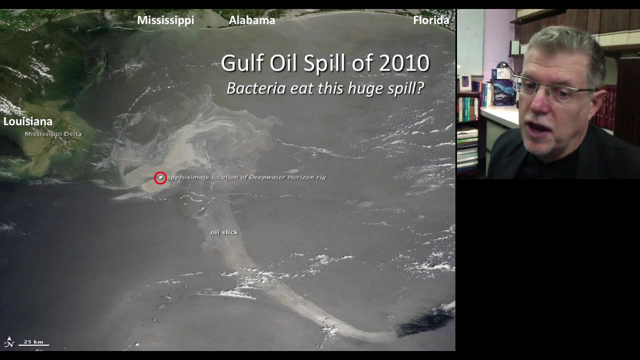 Now I want to give you an example of how microbes, their numbers, their presence everywhere- can really make a difference in terms of bioremediation- In this case, not engineered, but a naturally occurring bioremediation. So in 2010,, there was an enormous oil spill off the coast of 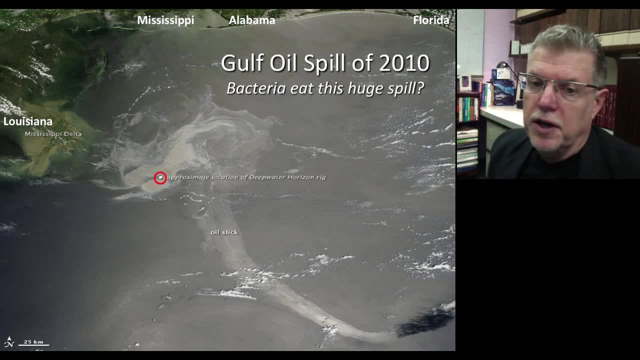 the United States. at an oil platform, It exploded and the oil was spewing into the Gulf of Mexico, So this was something that people were very alarmed about, and many people thought that this was going to cause environmental distress for years or even decades And in 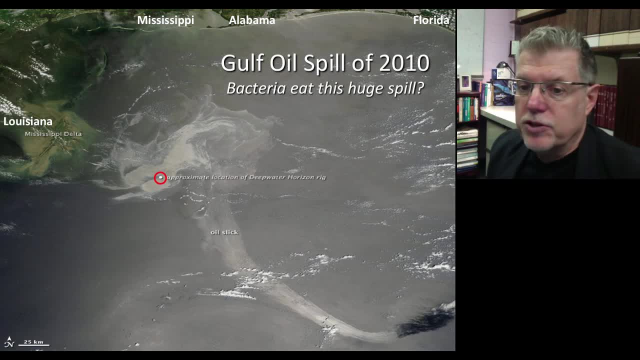 fact, a year later, there were many beaches that looked very clean and the water was much clearer. So what happened? Well, it was: They figured out that there were bacteria in the Gulf of Mexico that were naturally good at eating oil- some because there were many oil seeps in the Gulf of Mexico. So they 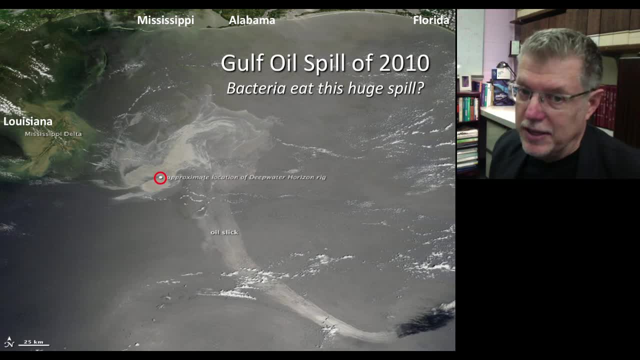 had gotten adapted and evolved to handle that oil, to eat that oil, And then over time they- in really a very short time- they proliferated and ate a great preponderance of the oil that was there. So we're interested in this. How do they do this? 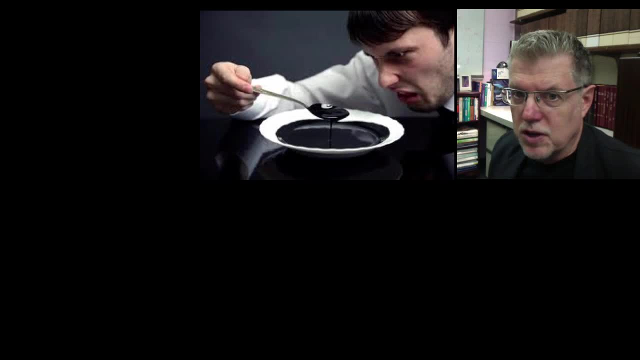 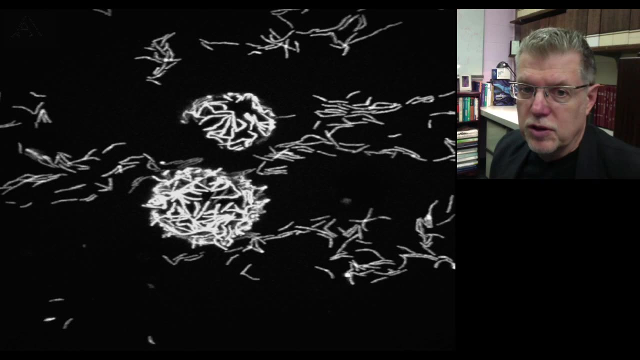 I mean, oil does not seem very palatable to us, but to bacteria they, in fact some of them, will adhere to the oil droplets, basically eat the alkanes, the single ring aromatics, the polycyclic aromatics, and they do this very efficiently. 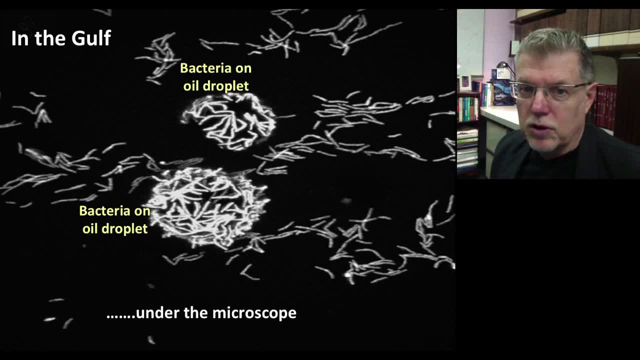 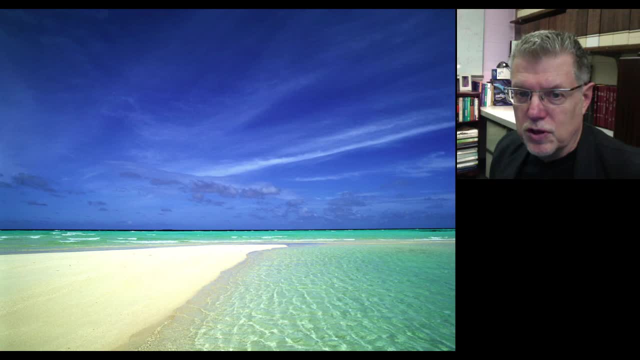 And, as I said, this is what it might look like under a microscope in a light field image. And, as I said, this is what many of beaches in the Gulf of Mexico look like, because of this enormous capacity of microbes to eat huge amounts of material. 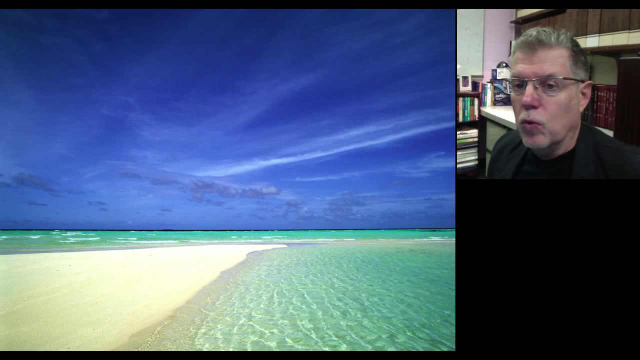 So we'd like to use this. So one way that humans use this is to study the biochemistry, the microbiology of the organisms that eat these, both natural products like oil, as well as industrial chemicals, And a lot of that information has been compiled over a long period of time, And we did this, working myself and Professor Linda Ellis. 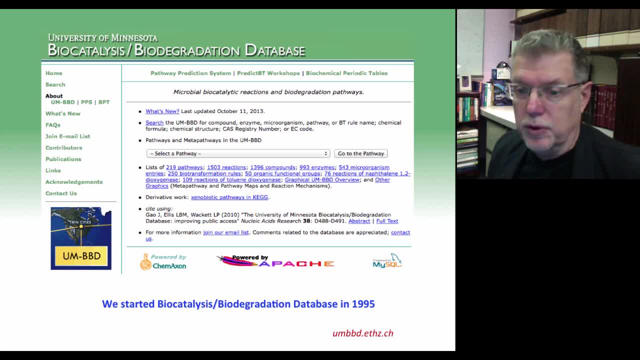 That's still going on. We started 18 years ago, or 19 years ago now, the Biocatalysis Biodegradation Database. So we compiled information not just from research here at Minnesota but from all around the world- many researchers over many decades- to better understand how microbes will degrade all different types of organic chemicals. 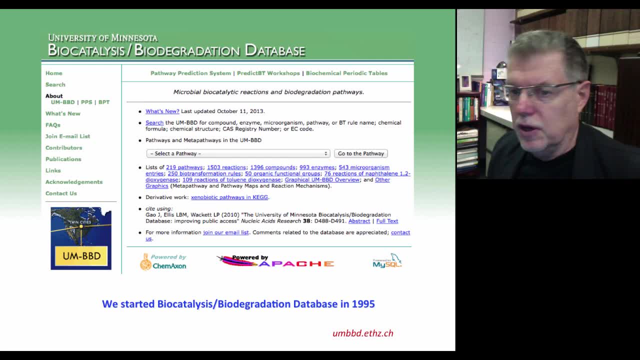 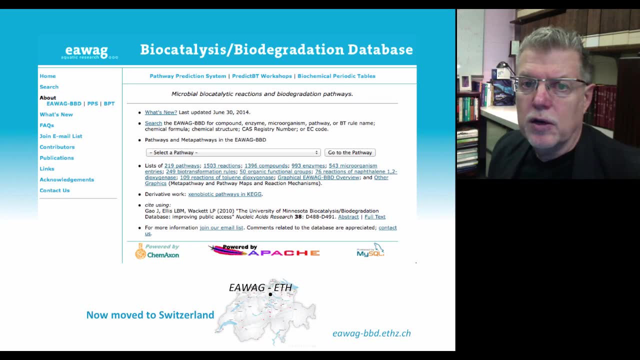 And this database has now been taken over and it's now maintained And in Zurich, Switzerland, where it's called the Eawog Biocatalysis Biodegradation Database, and the database is continuing to develop and we're very happy to see continuing developments and we hope this will continue for many, many years. 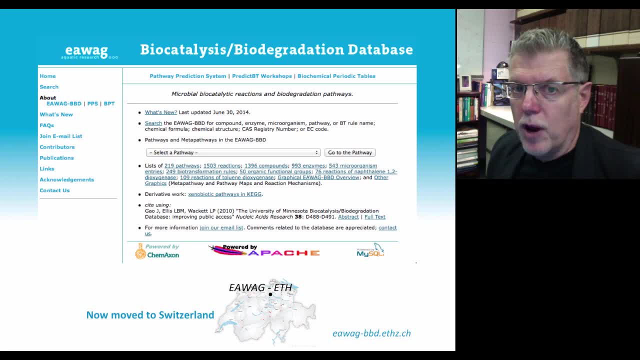 Now there's another feature of this database whereby we can use the accrued knowledge for many years of biodegradation research To then extract rules and knowledge that can be used to predict the biodegradation of chemicals that have not yet been tested. Now this is important. Think about chemicals are being new, ones are being made all the time by industry for all kinds of uses- as pesticides, drugs. 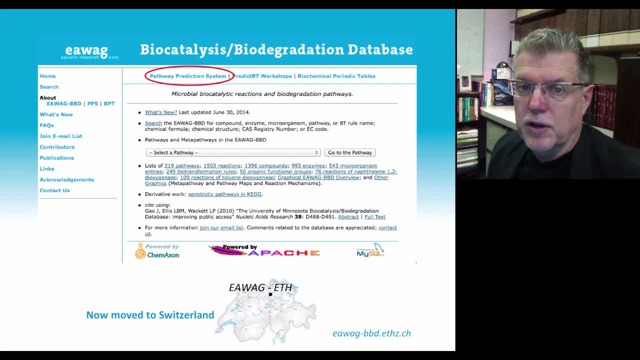 And we would like to know what their fate is in the environment. So we use this pathway prediction system that we've developed, and many people, thousands of people, have used this around the world, And let me show you a little bit about how it works. 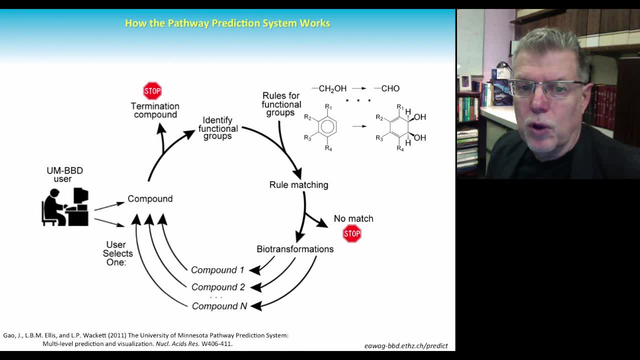 So generally the user will enter a compound. they can draw this with an easy drawing package And then press go and the system will start predicting, putting rules onto the structure and then predicting biodegradation reactions and then string those together to make pathways. 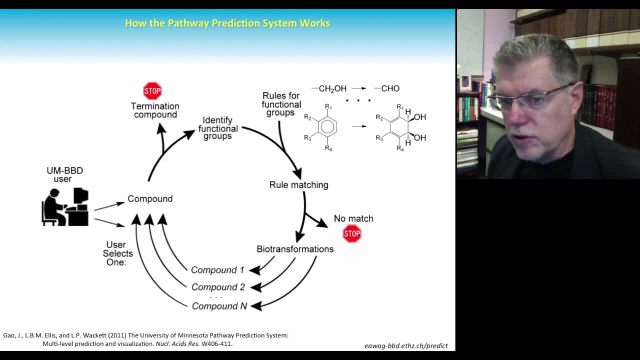 We've published extensively on this, So if you want to know more how this works, you can look up some of the many papers that have been published on this. Now, just to give you an example of how this is used in. one particular example I'm going to show you is with the chemical atrazine. 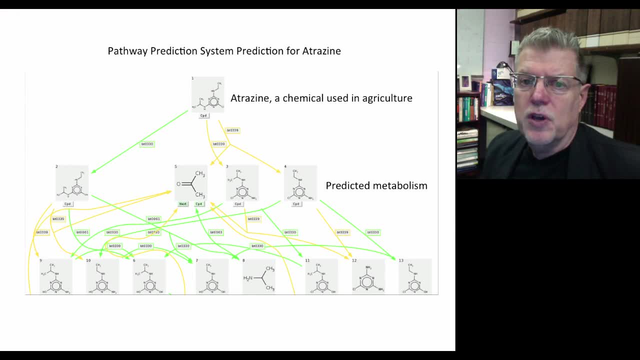 That's shown on the next slide. In this case it's a chemical that's used in agriculture to kill weeds, And you can see there's a lot of lines going in from different metabolites. So atrazine is at the top, the parent compound. 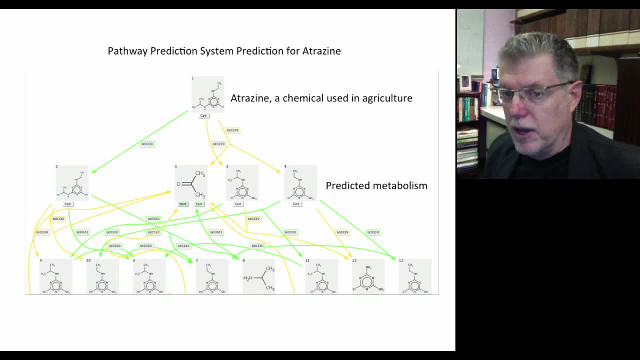 Then it makes, can make various products And those in turn can make products. And you can see that these pathways are overlapping, So it can get quite complex, But we've been able to also put priorities. You see, the green lines- The green lines would be the most likely pathways. 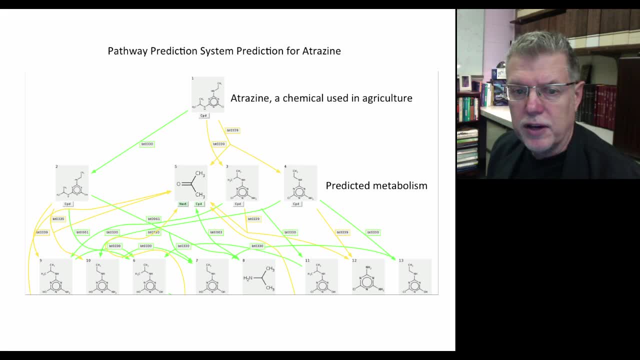 Based on the current knowledge. So if you follow the green, you'd see you just go down one pathway And that's a pathway that's been well established in nature. So the prediction system works quite well. So let's see what has been known from experimental work. 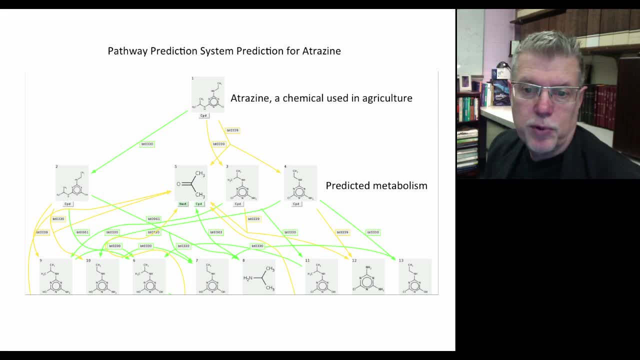 So this is computational prediction, which could be applied in this case to. it's applied to atrazine, a known compound for biodegradation, But it can be applied to millions of chemicals, even ones that are newly underdeveloped, And so it's used a lot by industry, by government regulatory agencies, to get an idea of the fate of chemicals in the environment. 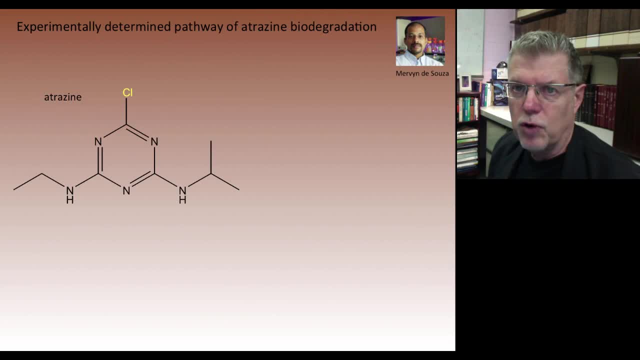 Let's see how atrazine is known to be degraded. This was worked out first by Mervin DeSosa, working in my laboratory, And he showed that what bacteria do is start starting with atrazine. And he showed that what bacteria do is start starting with atrazine. 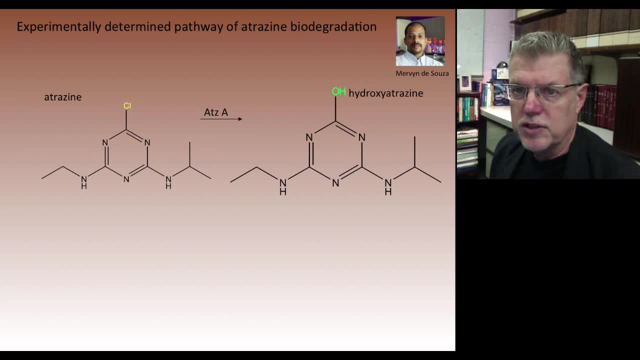 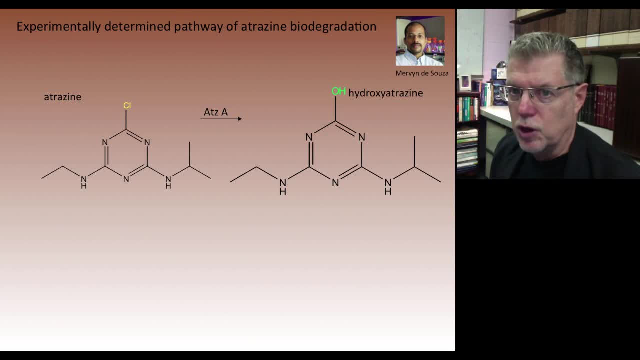 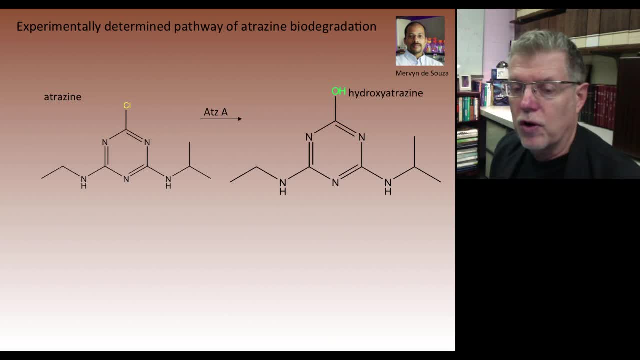 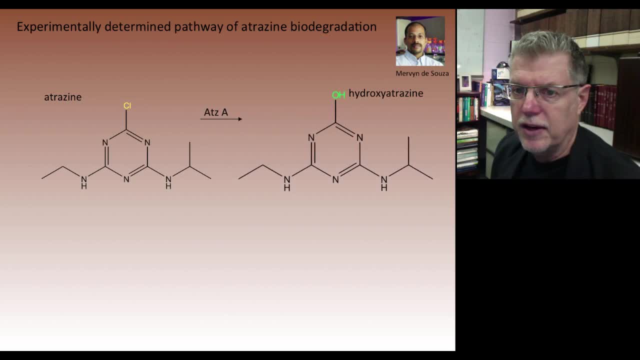 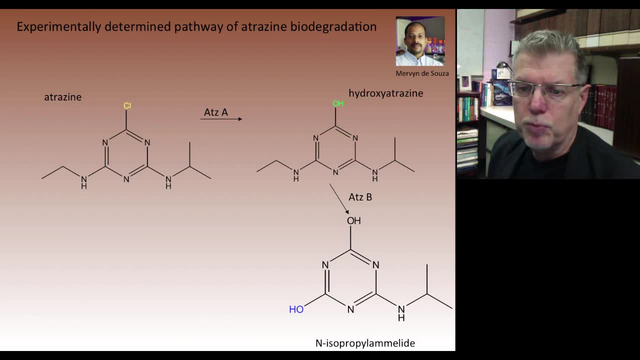 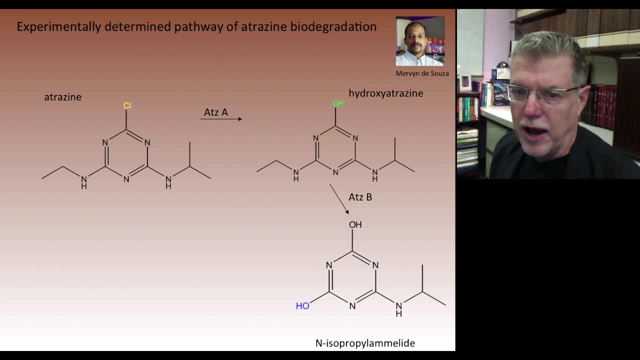 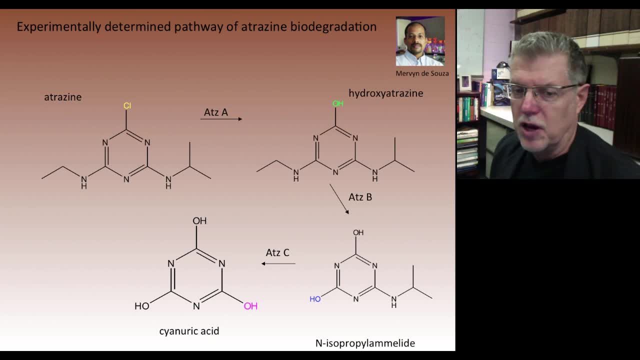 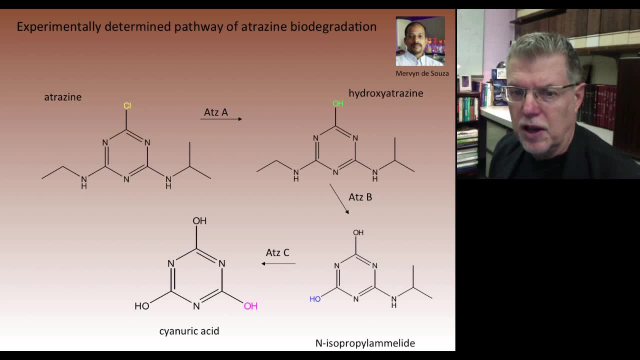 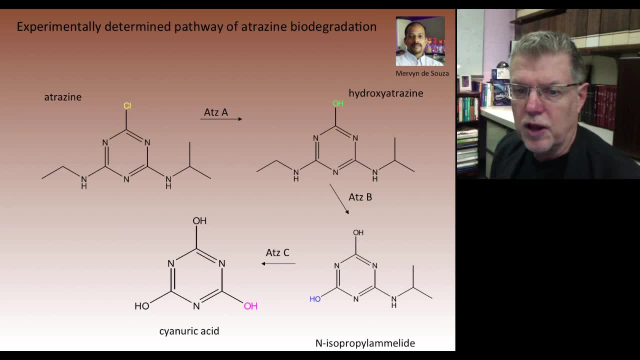 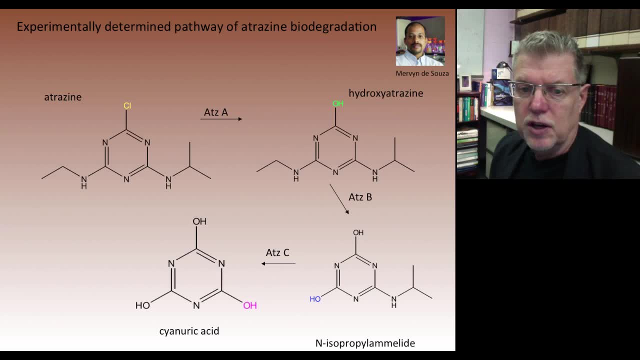 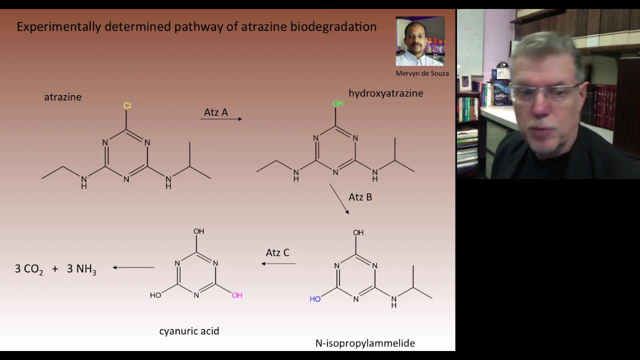 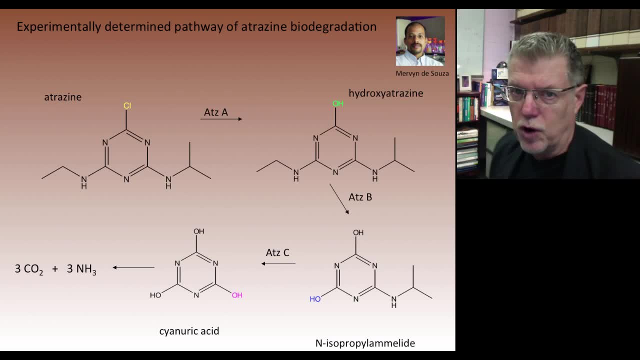 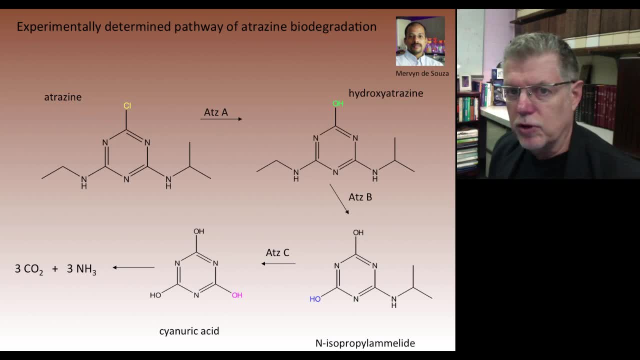 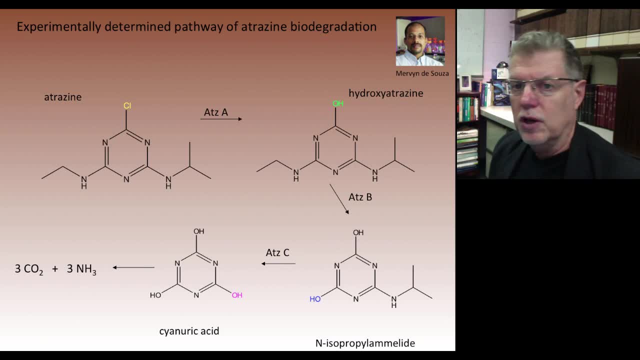 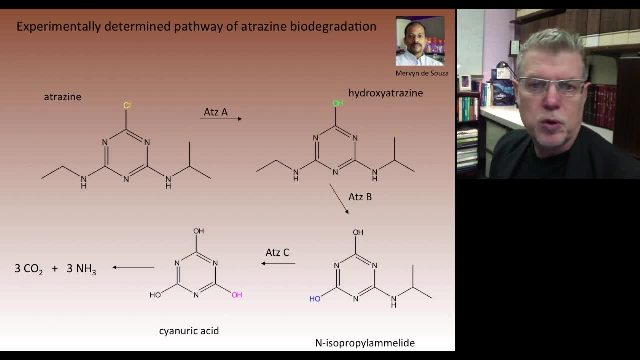 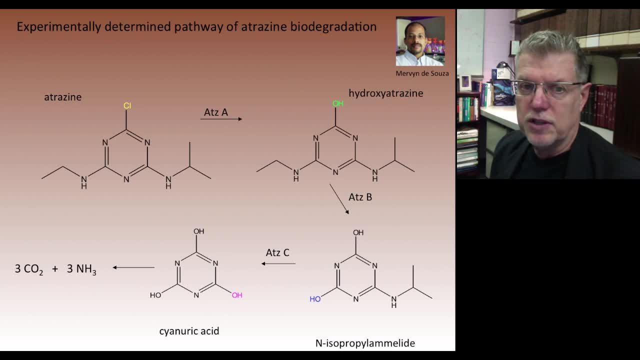 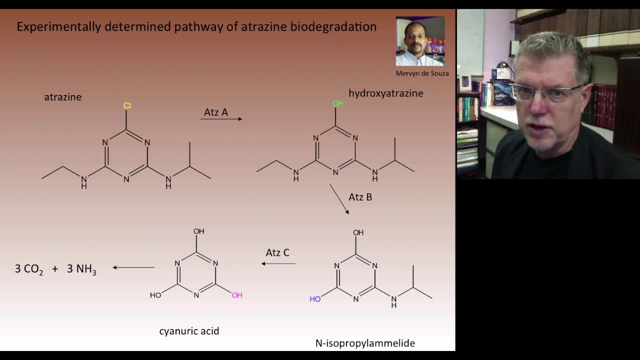 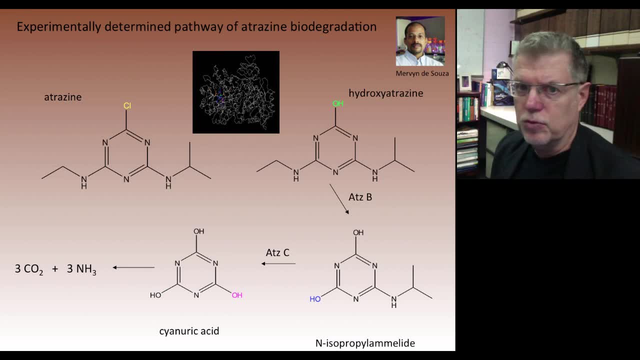 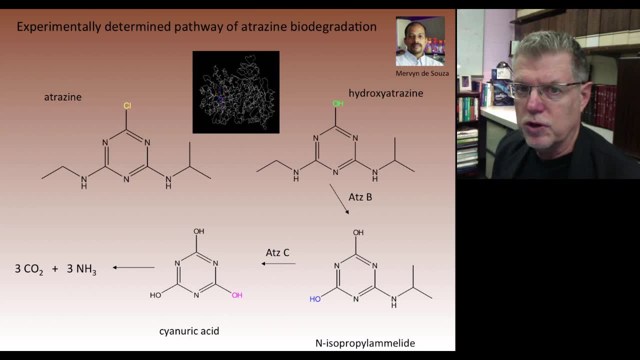 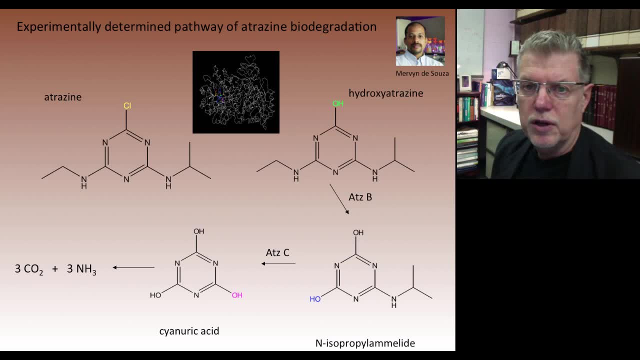 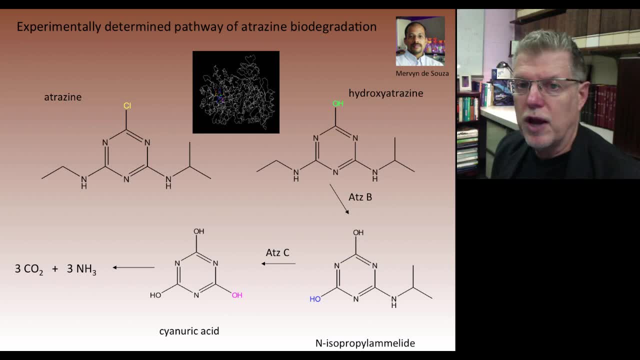 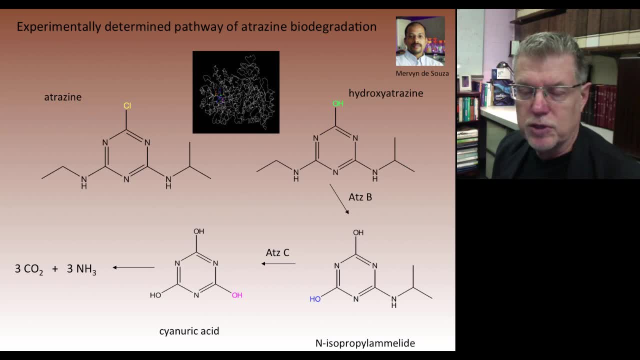 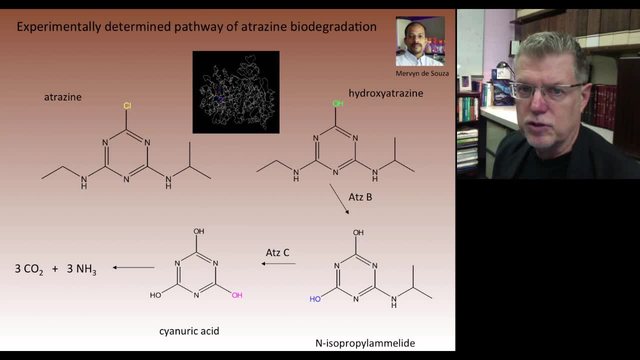 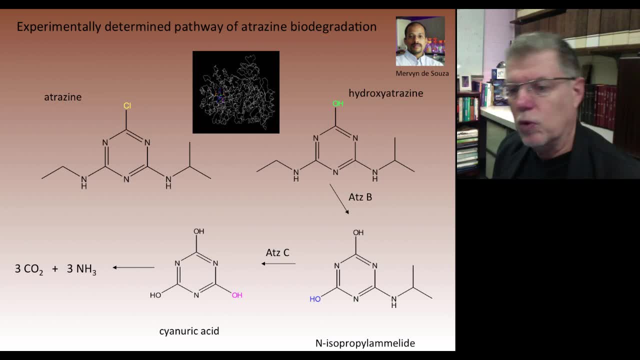 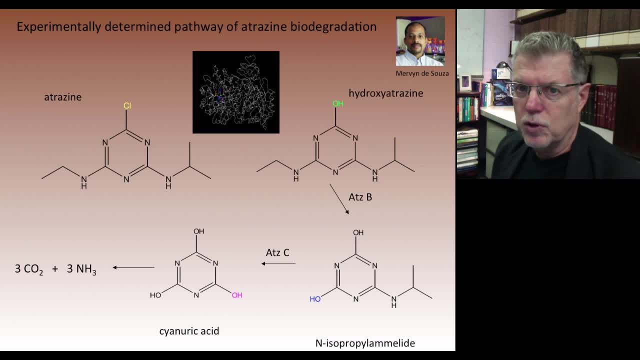 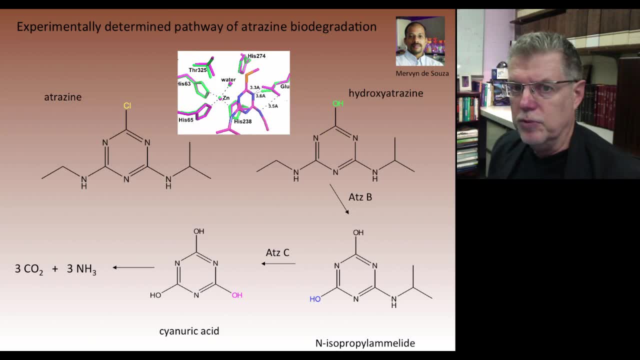 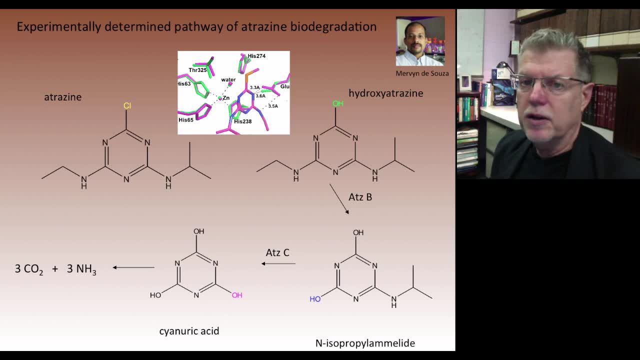 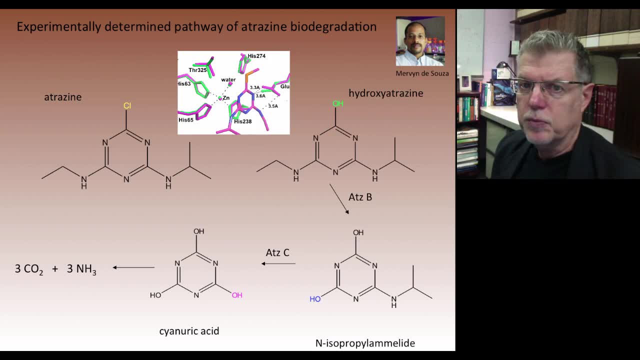 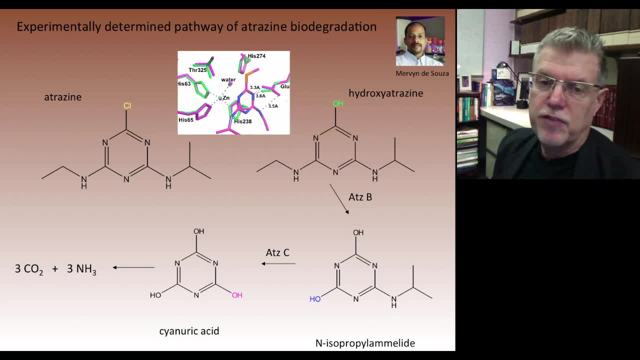 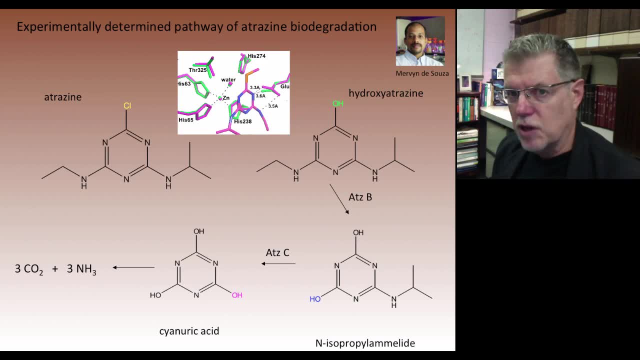 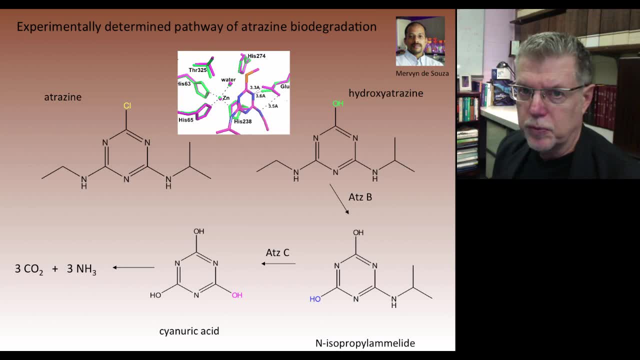 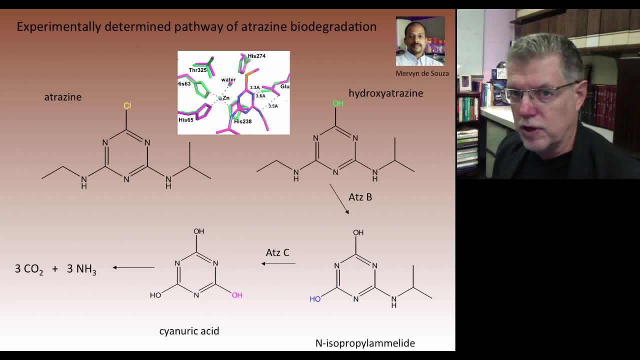 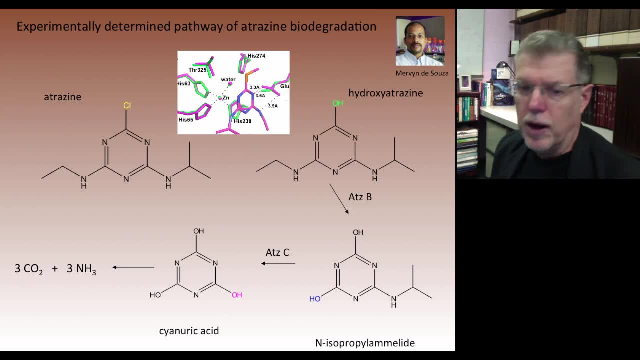 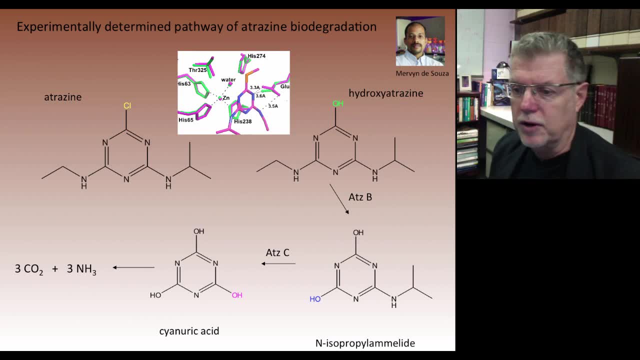 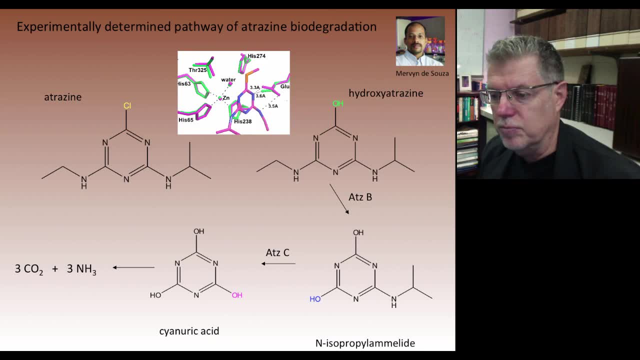 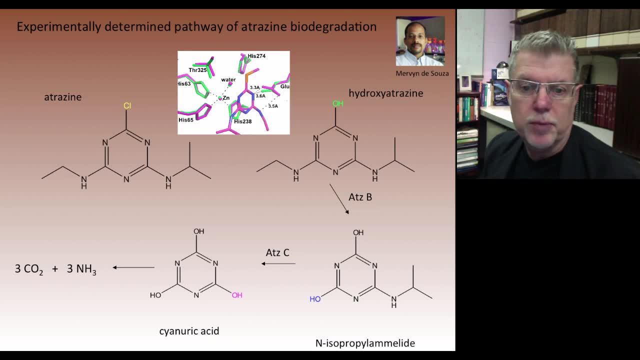 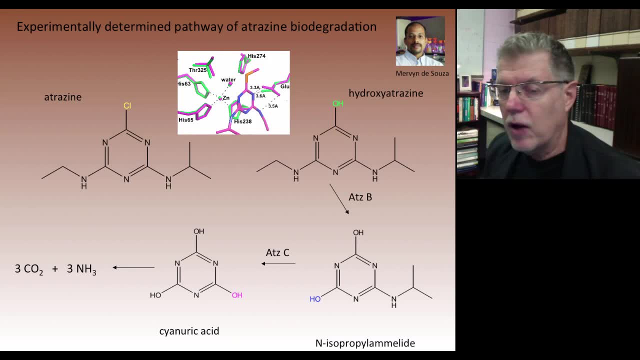 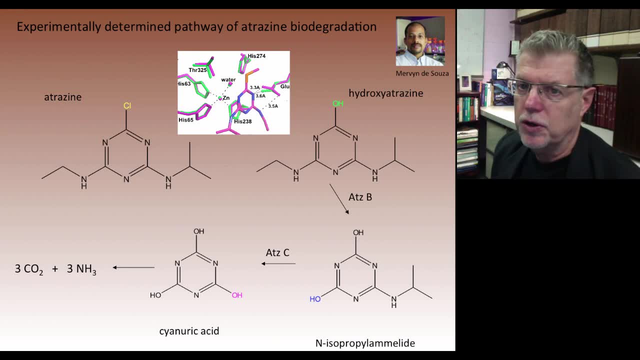 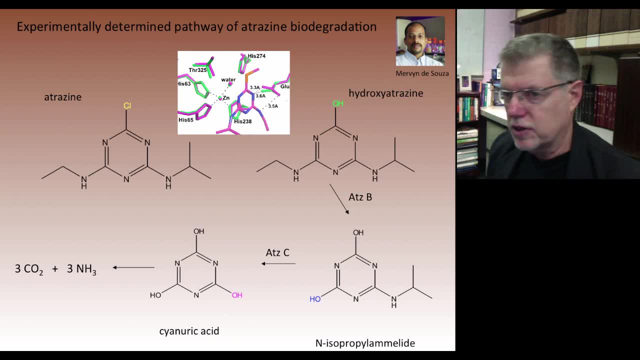 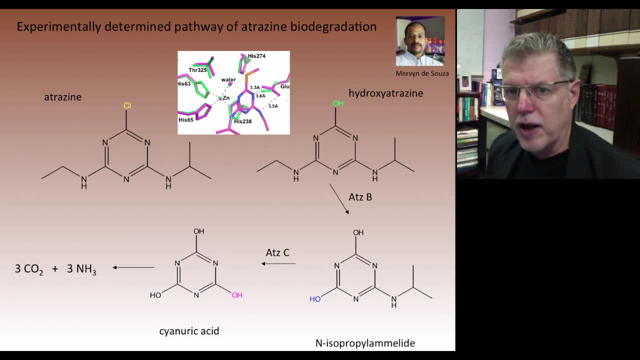 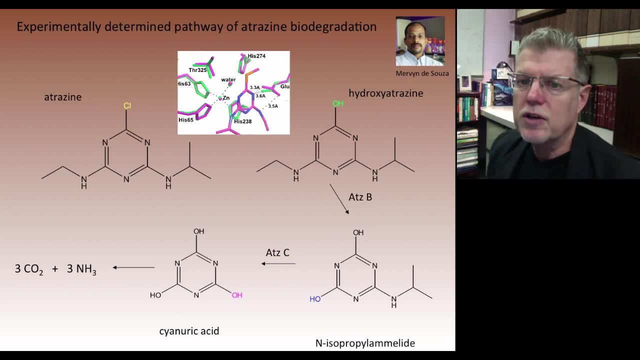 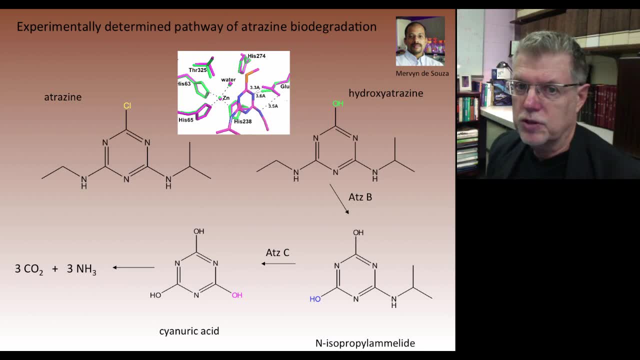 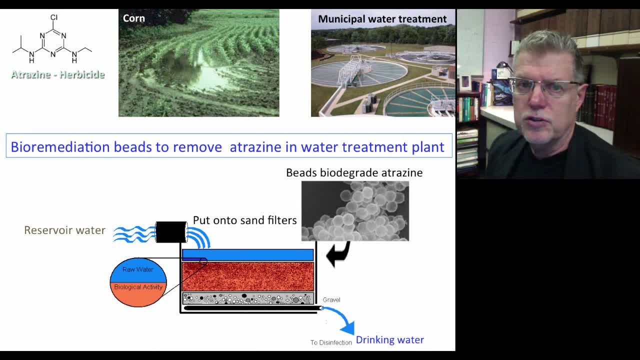 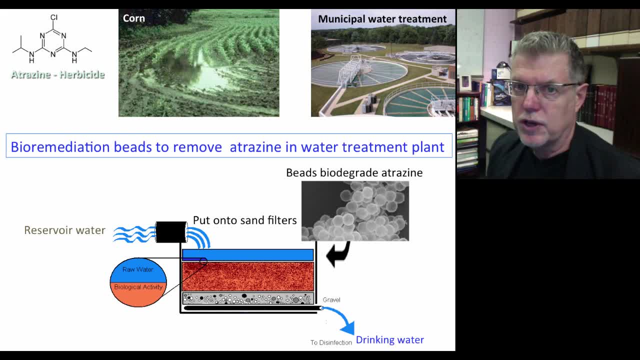 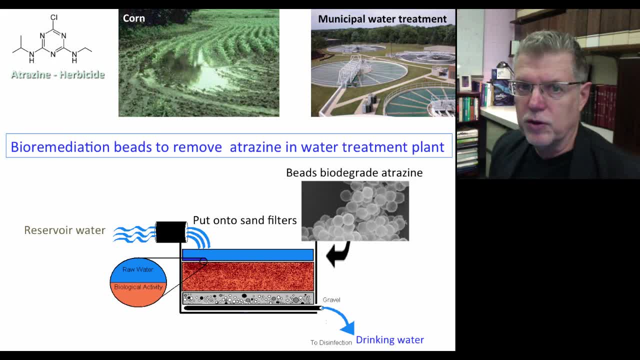 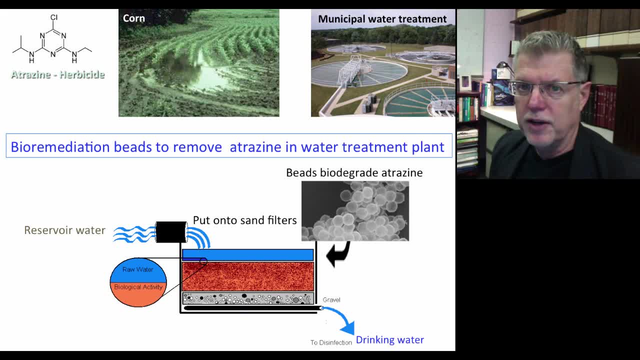 And he showed that what bacteria do is start starting with atrazine. in the year when atrazine is applied, you could potentially get some running off the field into streams and rivers. it might make its way to municipal water treatment plants and then we felt that we could use then this atrazine. 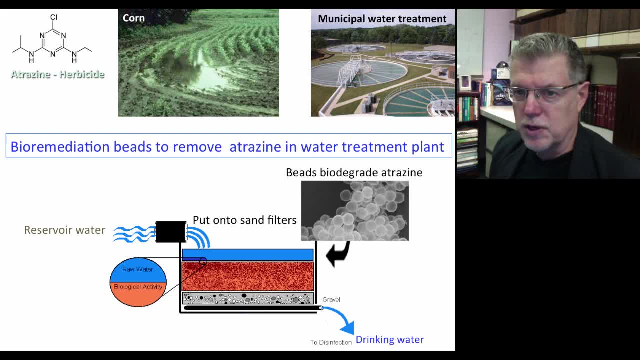 degradation mechanism in a biological system, in an engineered system in beads that would then be put onto a sand bed, filter the water then. this is something that's, in normal water treatment plants, very common, and so, as the water goes through the filter, it's also going through the beads and that's it's passing. 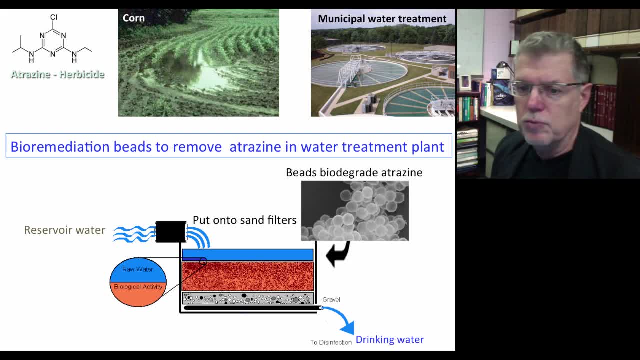 by the atrazine is degraded and so it's removed, and then it's not present in the drinking water. so what about these beads these are? you know what are they? these are not naturally occurring. this is where the organism in the enzyme is put into this bead. 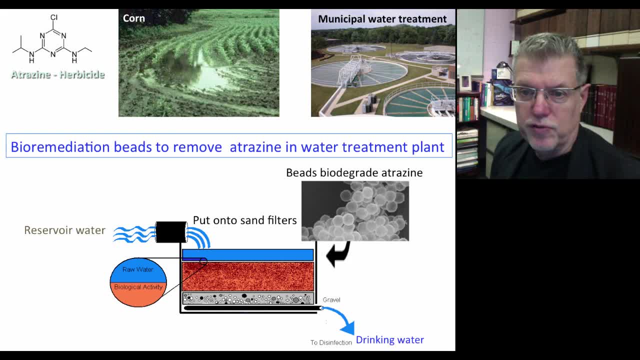 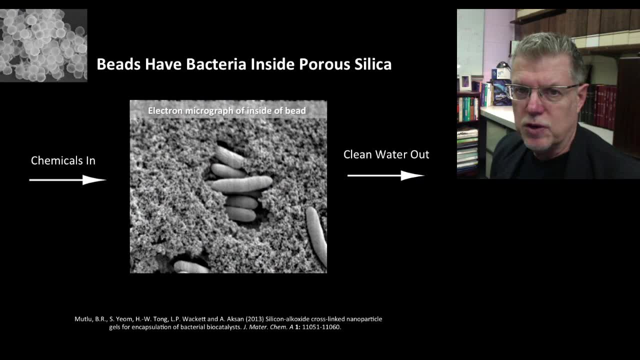 so that it's not released And also it's preserved in a more stabilized form. But how do we make these? So let me show you what these beads are. So the beads have bacteria inside them and it's made of porous silica. So this is in the middle as an electron micrograph. 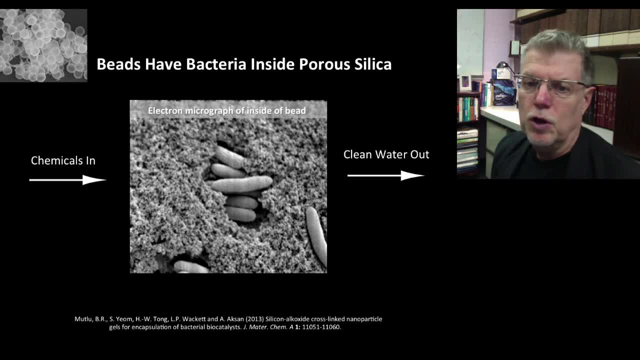 that shows you this kind of porous, spongy structure with the bacterial cells that are trapped. So this has been broken apart. Normally the bacteria are completely surrounded by the silica and so they can't get out, but what chemicals and water get in? 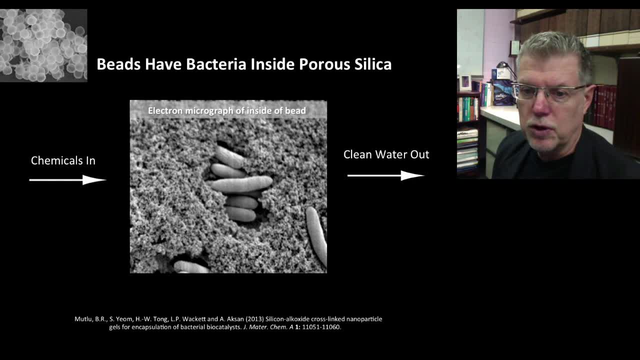 the water then gets cleaned, And we've published again on this, so you can look up some of our several publications if you wanna learn more about how we make these. But I'll just tell you briefly how we make these because, remember, the bacteria are trapped inside. 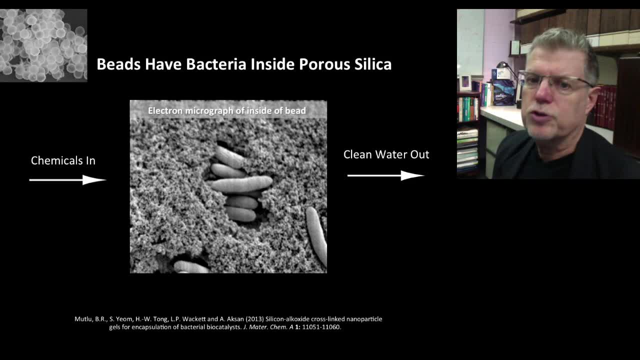 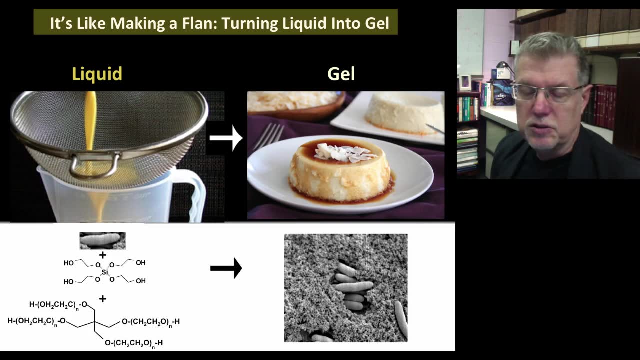 they're not just stuck onto the surface. So how do we make a structure like this? Well, it turns out. it starts out, it's like it's a liquid, So we make it when we make it into a gel. So this would be like making a certain kind of cake, right? 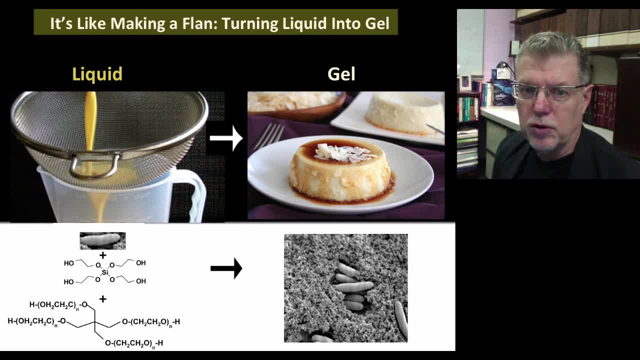 Where you have a liquid material that you then cook and make it into a gelled food that you might eat. In the same way, we have now these silica precursors, these silicon alkoxides. we mix with the bacteria and we may also mix some other materials. 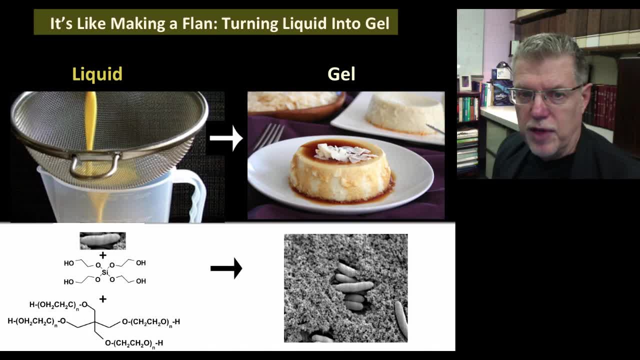 polymers, and then that liquid gels in the system that we make, And then the polymer in the sense forms around the bacteria. So the bacteria get trapped or encapsulated within the matrix and then it can be used. Now the difference between the cooking example. 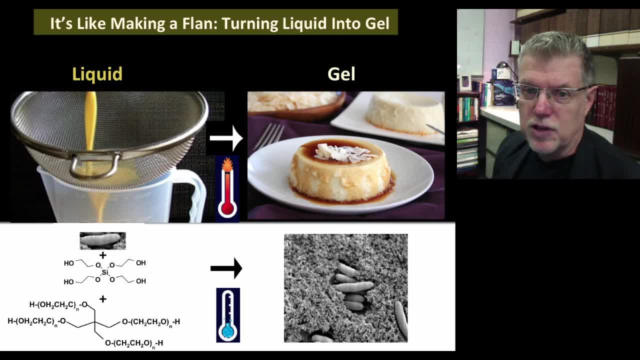 and our manufacturing example is that the cooking has to occur at high temperature And of course we wanna preserve the enzymes, So we use materials that we can encapsulate the bacteria at a room temperature. So it's a very gentle procedure which is essential now for keeping the organism alive. 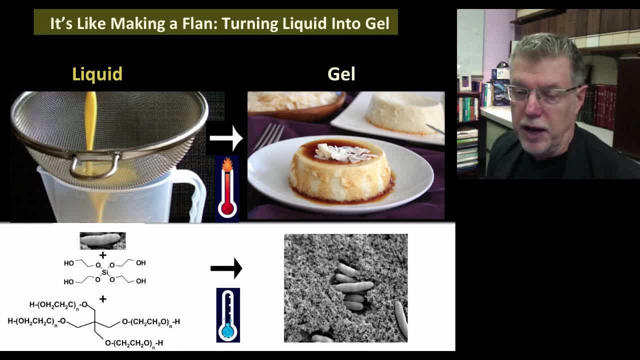 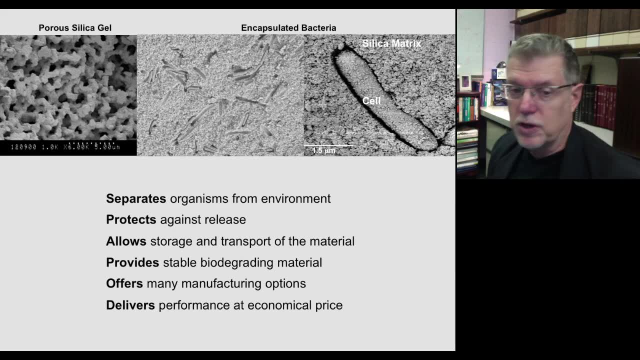 All right, let's see another way, an application, another way we can make materials like this. But first let's say I'm just gonna tell you briefly the values of materials. So when we're making this type of material one, it separates the organism from the environment. 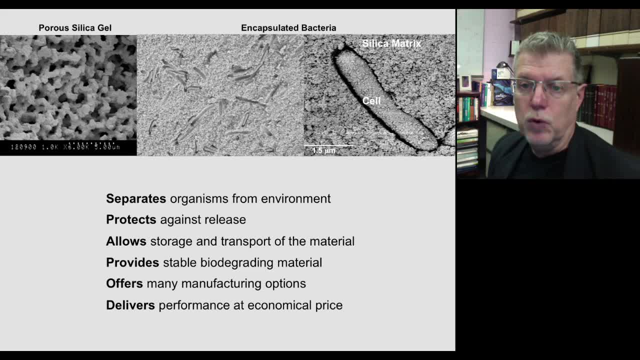 It protects the bacteria against releasing, So we wanna keep them contained. We don't want them to go through the filter and get diluted. It allows storage and transport, So we make beads. They're dry, they can be shipped in containers And we've done this to different sites. 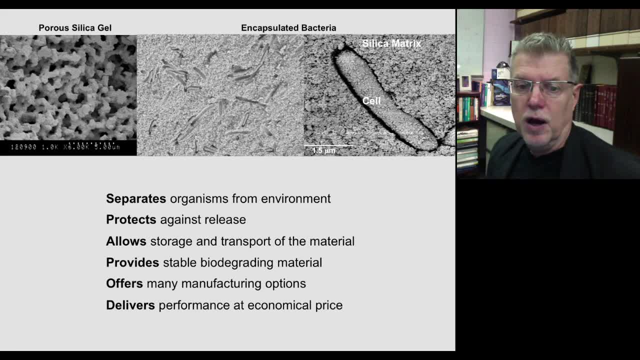 You can provide stable biodegrading material then for different applications. There's many manufacturing options. We make beads, but we've also made wafers and fibers, as you'll see, And also this material, the silica material, is fairly inexpensive. 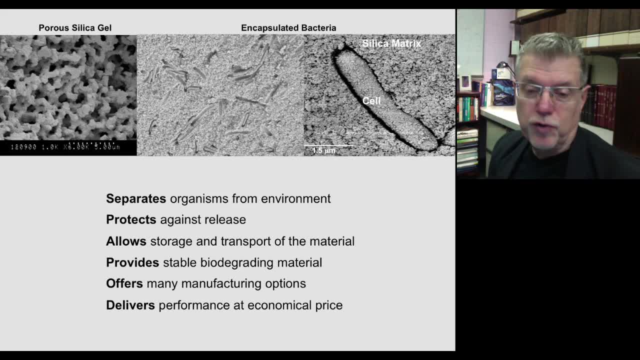 So we can make a material that's useful for bioremediation, but not at a very high price, which most people don't wanna pay. They wanna clean up an environment, but they usually wanna pay the least amount that they can to get the job done. 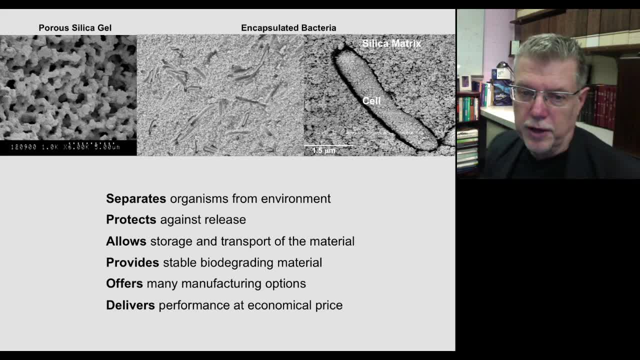 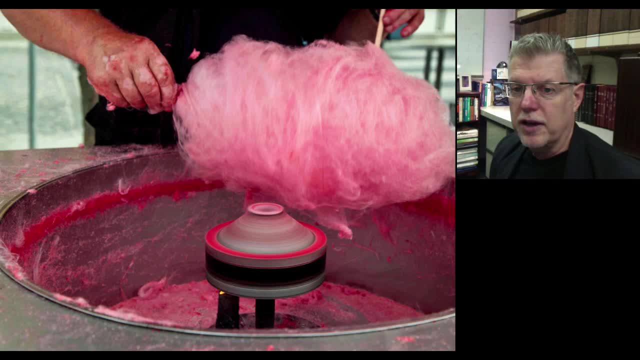 And this helps to do that Now, as I sort of indicated that we make another material, So this is more like something that you might see. This is called cotton candy. Some of you might've eaten cotton candy. It's basically a fiber of sugar. 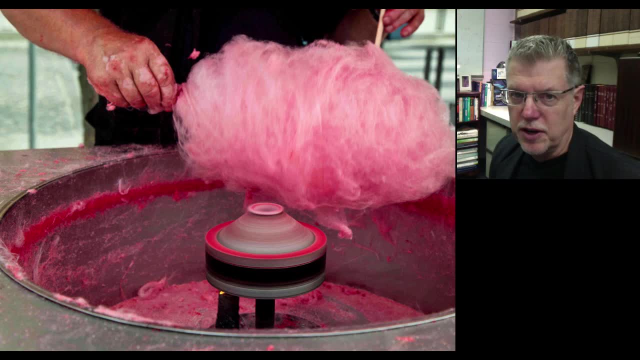 and then it's usually has some flavor and colorings in it And the process of doing this. there's a middle spinner that then basically jets out the sugar solution and then it forms these fibers. Well, we can actually do something similar with the silica material and bacteria. 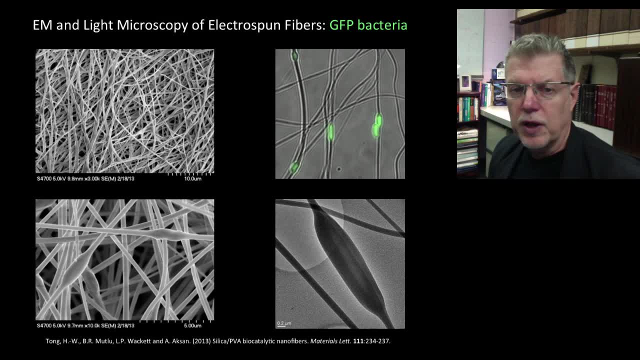 I'm gonna show you that here on the next slide There's a light microscopy images on the left- or actually in the upper right, I'm sorry- And then the others are electron microscope images. You can see how the fibers are very thin. 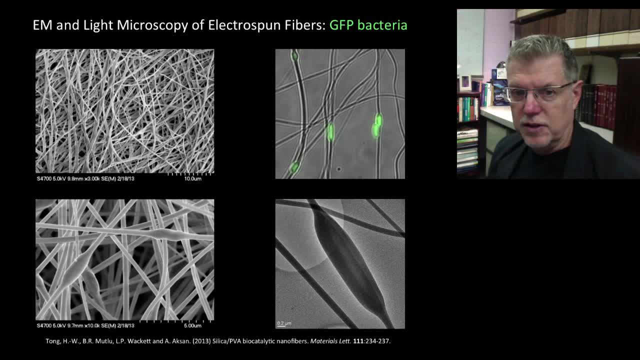 They're really nanofibers that then bow out around the bacteria that get encapsulated. In the upper right is a light micrograph and that's showing green fluorescent bacteria GFP that is inside the cell. So it's now fluorescent And it allows us to very nicely image the bacteria. 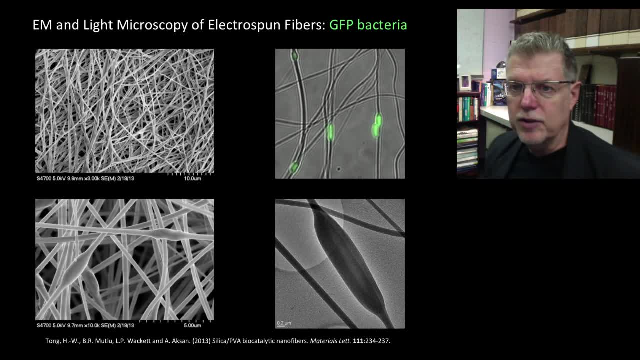 in this sort of glowing green color And you can see that they're stacked in the fibers. We can get a pretty high density now of bacteria in the fibers, So these would be like biocatalytic filters. You can use these. it almost looks like a cottony mesh. 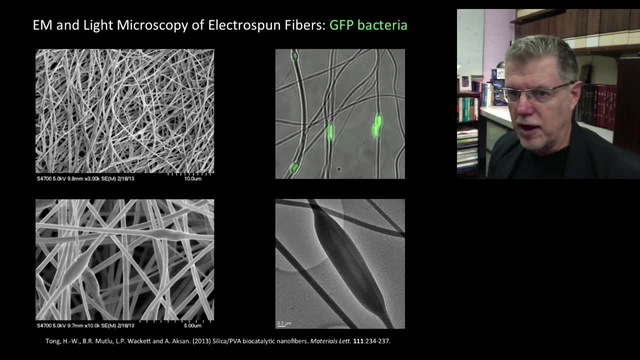 And you could pack this into a filter cartridge. You could have it for handling gases that are coming off through the filter, for example, or liquid. So we think there are many applications of this type of material as well, And so this is something we're actively working on. 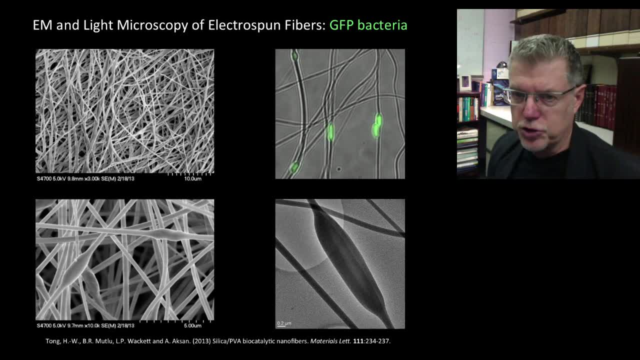 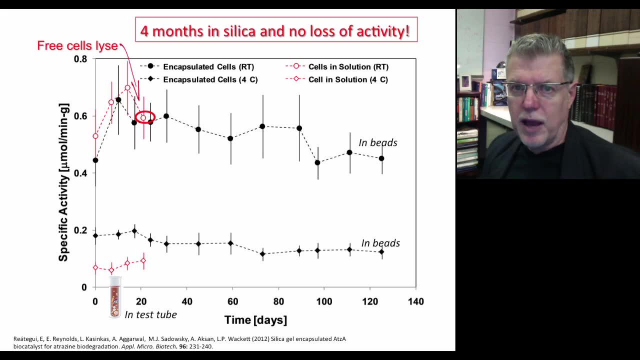 to promote biomediation applications. All right. so this illustrates one of the benefits of the encapsulation process. Here we have bacteria in the red With free cells. you get a good activity, but after about three weeks or so the cells are lysing and you largely lose activity. 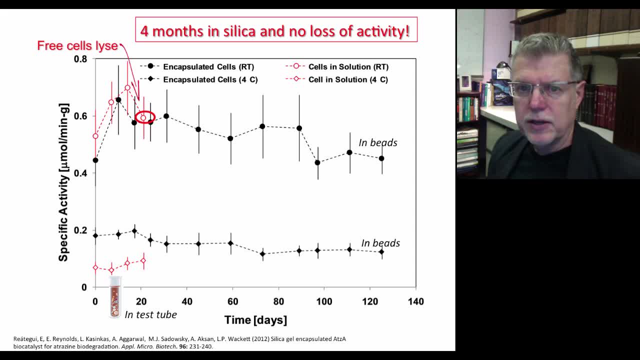 But you can see with the black points and the curves that in the beads the catalyst, in this case the atrazine degrading enzyme, stays active for a very long period of time, In this case four months, which is about as long actually. 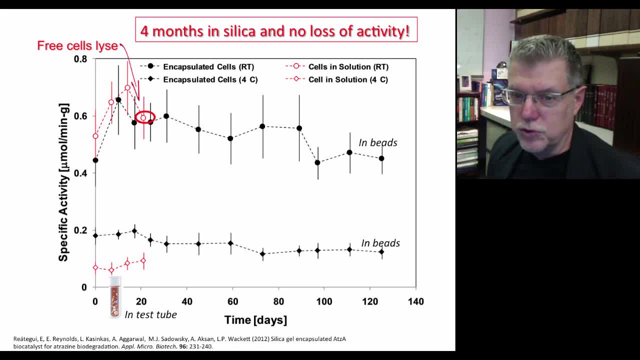 as the student doing the work took time points, So you got bored after that And you can see also: the top graph is at room temperature and the bottom is at four degrees centigrade And you can see that the bacteria in the beads behave. 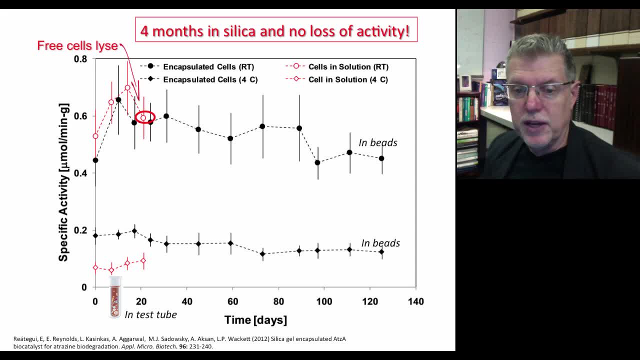 and perform better while they're inside the beads, And we think that this is because when the cells are encapsulated, they crack open a little bit and they become more porous to the chemical, in this case atrazine, so they actually show enhanced degradation rates. 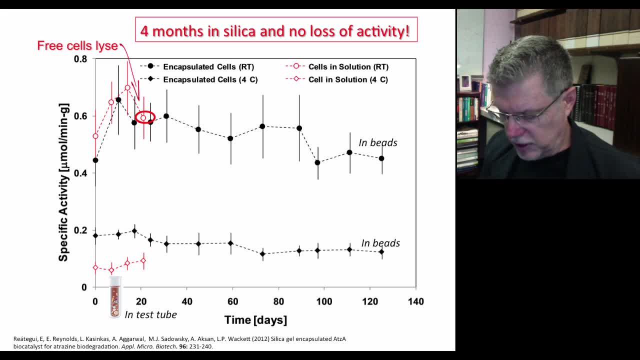 So this is an added benefit of the encapsulation process. All right, so I'm just going to tell you about a newer application, of how we want to expand the use of these materials and to biodegrade a much wider class of materials. So this just illustrates another spill. 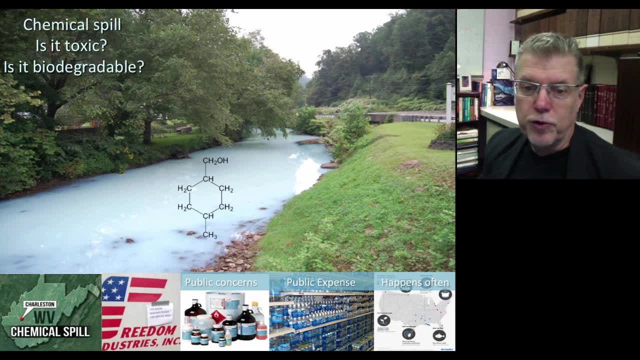 So chemical spills are hopefully not common, but they do occur And when they do we really depend on bacteria to clean it up. either just bacteria in natural ecosystems if they handle it, or in some cases we have to intervene and engineer systems. 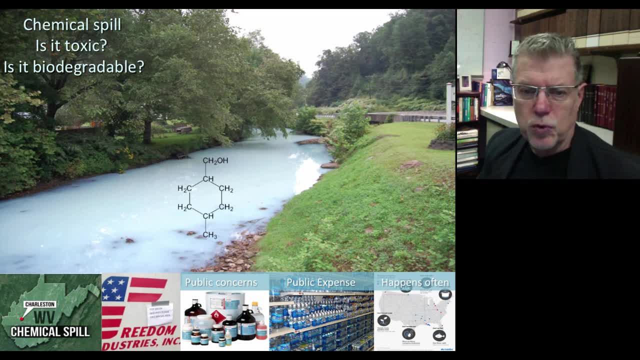 to clean up the chemical. In this case it was a coal cleaning chemical. This happened in the US, in the state of West Virginia. The structure of the chemical is shown And it just illustrates that this can be really damaging. The local waterways were closed. 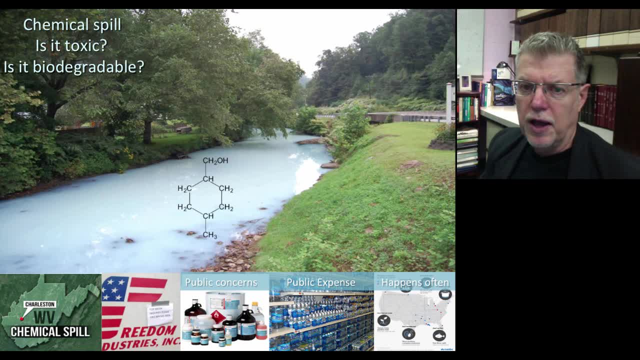 People couldn't shower, They had to bring in bottled water, And so we'd really like to be able to very widely predict the biodegradation of chemicals- something I told you a little bit about- but also then to be able to very quickly engineer systems. 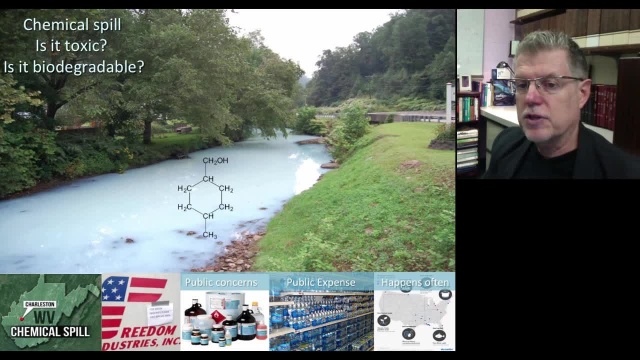 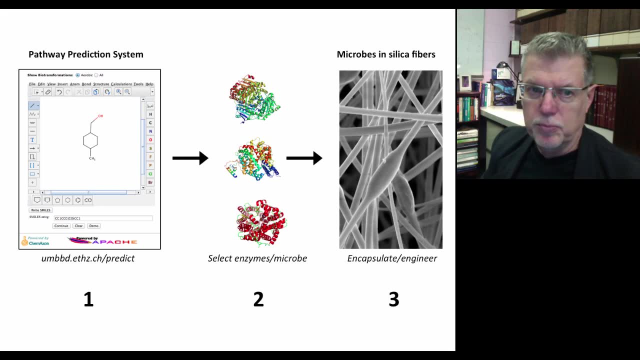 that could handle chemicals based on those predictions- And let me tell you briefly what we're doing about this area. So the idea would be to use something like the prediction system to, in this case, predict pathways, but also we're taking that further. 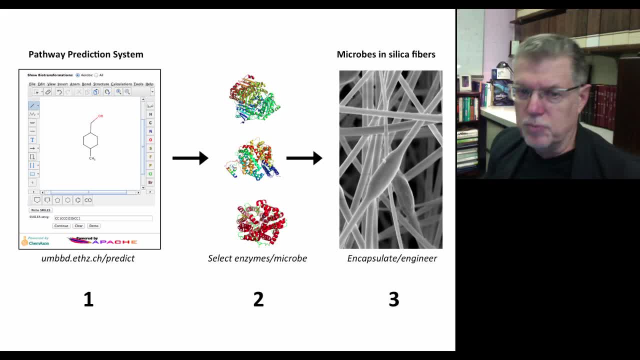 so that we could select the ideal enzymes and microorganisms that would degrade those chemicals, And then we could put those into silica microfibers that then could be deployed And with predictions, with computer work, with a lot of knowledge built up ahead of time. 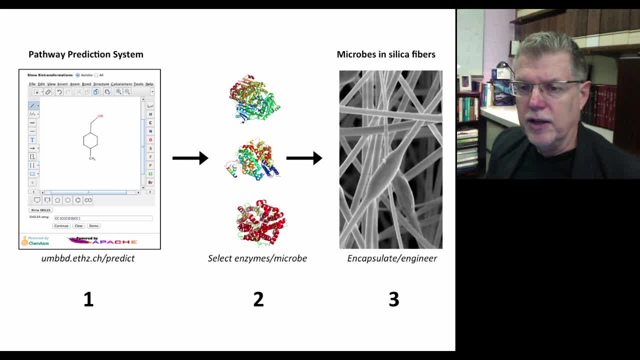 this is the kind of thing. then we could make a prediction and make a treatment agent very, very quickly, And that's the goal: to be able to do bioremediation much more effectively and much more quickly. So part of this is to understand. 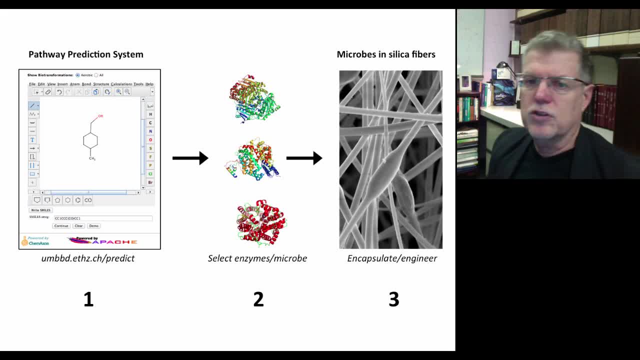 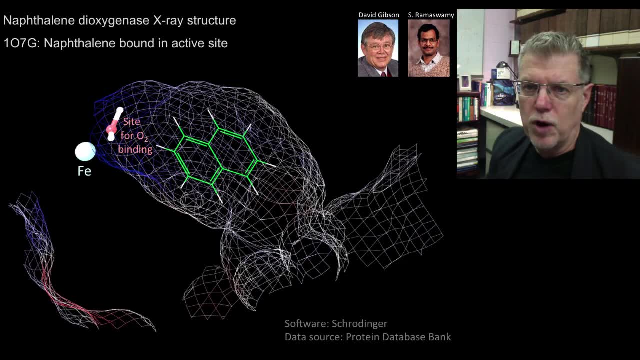 how different chemicals are degraded. And to do that we're looking at the structures of many biodegrading enzymes to see the range of chemicals that they will biodegrade. So this is one such chemical or one such enzyme: naphthalene dioxygenase. 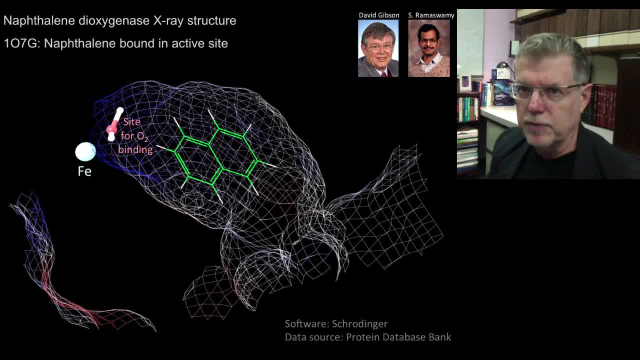 and you see the chemical naphthalene bound in the active site. And this is possible due to the work of David Gibson, who first purified and studied these enzymes, and S Ramaswamy, who deduced the X-ray structure of this enzyme. 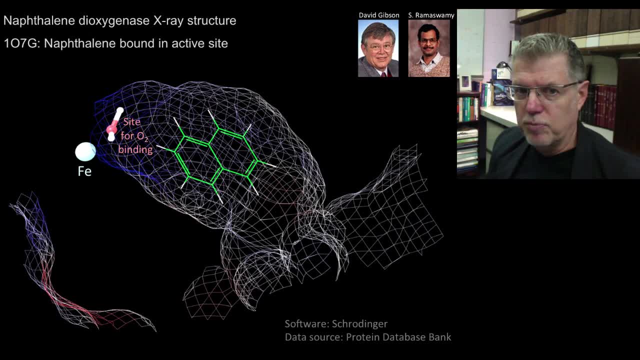 and a number of related enzymes, And so from the knowledge that's generated on the structure and the mechanism of these enzymes, we can use now software and dock other chemicals into the active site that might fit and react by getting near the iron, and then also that's the site where oxygen would bind. 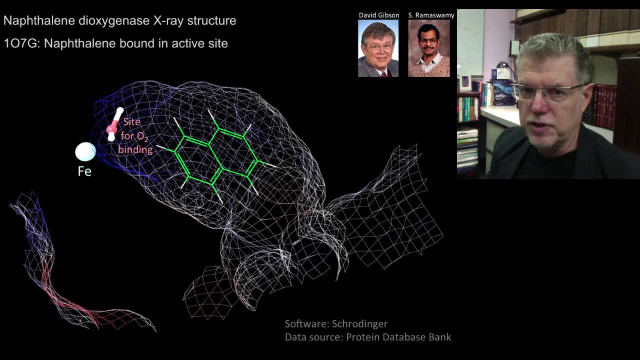 and be activated for reaction with these different aromatic molecules. So in fact, the Nobel Prize in Chemistry was awarded last year for this type of work to basically use computational methods for predicting chemical and biochemical reactions. So it's considered a very important tool that is being used much more widely now. 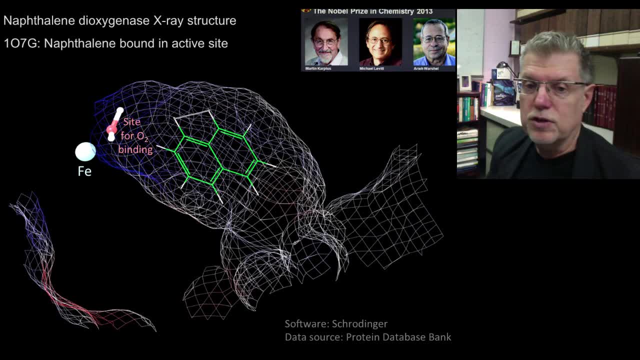 in chemistry and biochemistry and we seek to use this for biodegradation. So you see another chemical docked in the active site. now It has three rings instead of the two of naphthalene, and this fits in and we would predict it gets oxygenated. 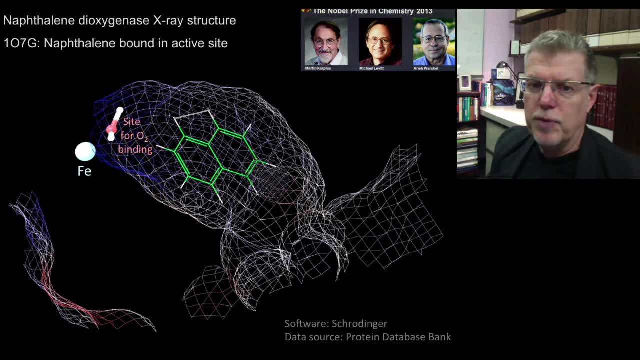 and it turns out experimentally that it does. Well, what about if you now have a fourth ring? Well, it turns out that would also fit into the active site of naphthalene dioxygenase and would nicely get oxygenated. So we can use sort of the go-between. 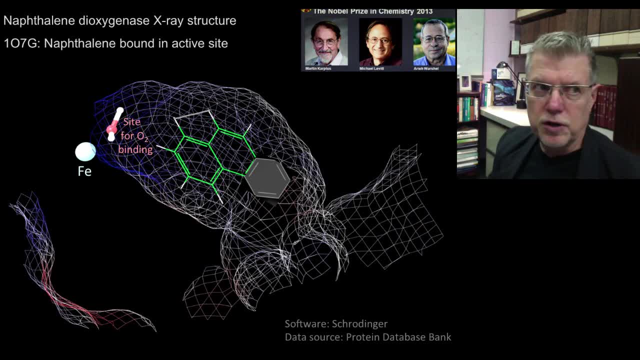 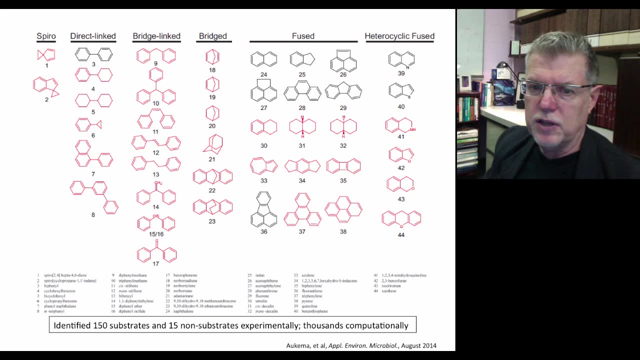 of computational prediction, experimental validation, so that we can over time really greatly extend the use we feel of computational predictions. Let me show you some of the experiments that have been done to complement this work, For example with this enzyme, naphthalene dioxygenase. 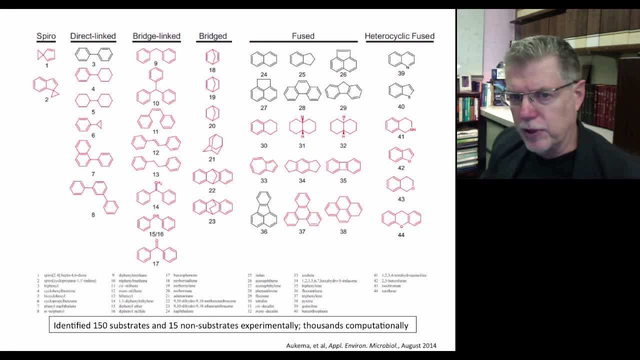 we just published recently that naphthalene dioxygenase will work on all of these aromatic ring structures, many of them shown here in this graphic. So it's a very broad specificity enzyme. It has a very nonspecific hydrophobic active site. 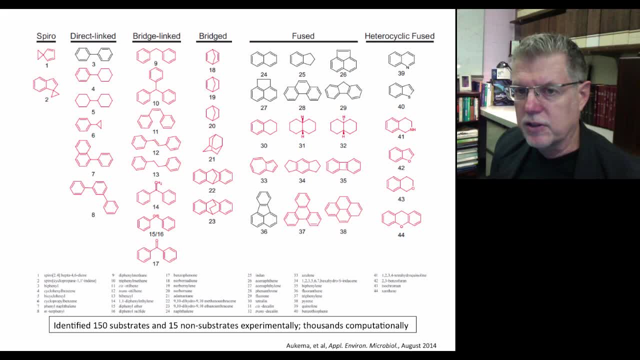 and there's quite a number of biodegradative enzymes that are like this, and a number of them have X-ray structures. So we feel that this approach with naphthalene dioxygenase can be greatly extended in order to do better bioremediation. 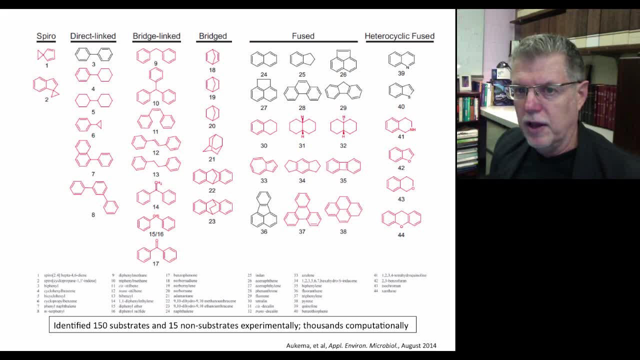 in the future to do it in a much more predictive way and to very much more quickly, when there's a spill, when there's a need to treat a certain chemical, that we can very quickly assemble the existing knowledge, make computational predictions. 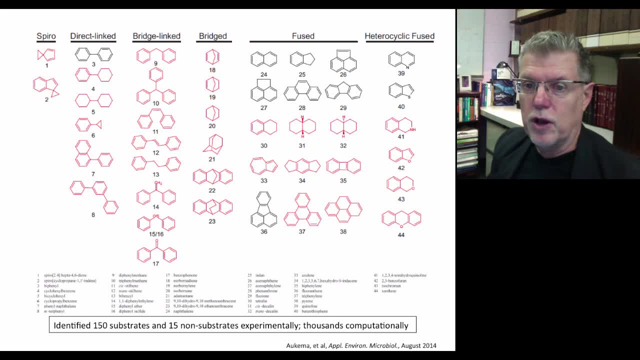 and then go and do something about the situation very, very quickly. So that's a lot of our research now and where we think it's heading. So why is this important? Well, I think many of you know that water is, you know, clean water especially. 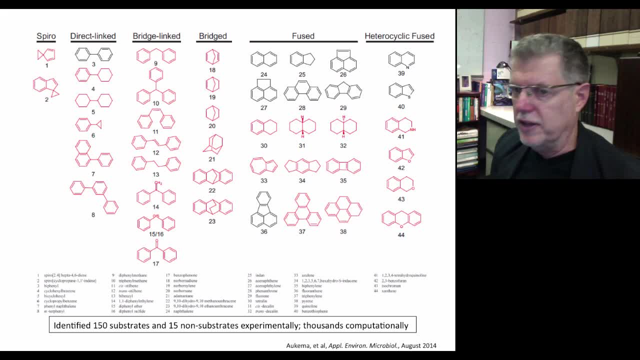 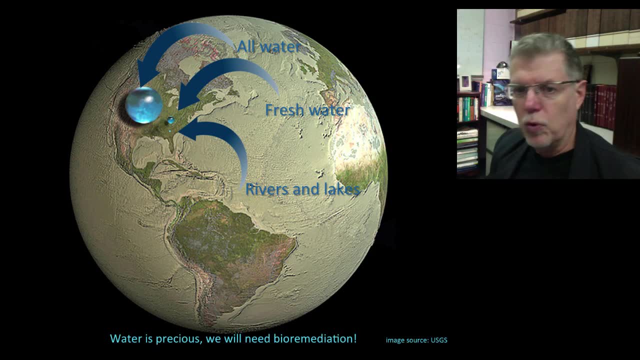 that for drinking water, for agriculture, for industry, for all applications- is becoming harder to come by. So one really beautiful way to look at this- this is from the United States Geological Service website- that what this person did, who made this graphic. 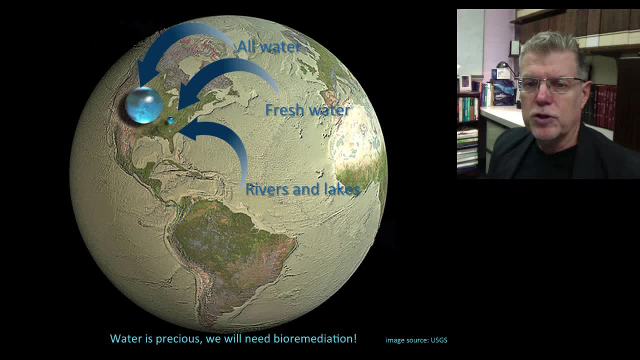 was to basically calculate how much water there is on Earth and then make it into spheres that would be proportional now to the actual amount of water, and then to place that on a globe So you can really get a sense of how precious water is. 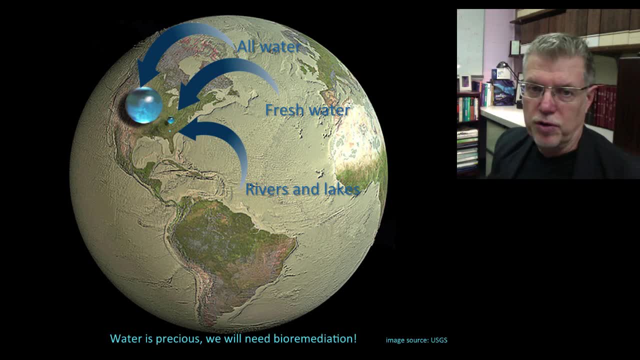 So you can see that the largest sphere is all water on Earth, including all the ocean water. The smaller sphere, in the middle, is just the fresh water, And then the smallest sphere, which is very, very tiny on a global scale, represents all the water. 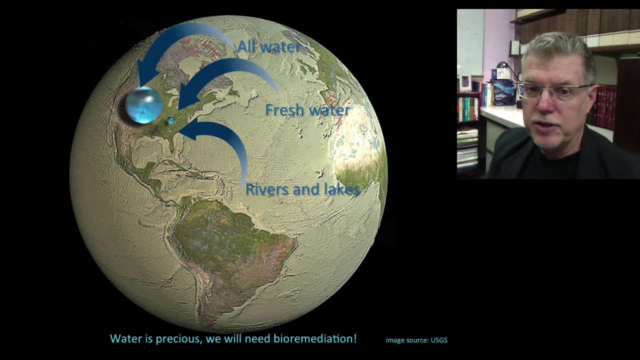 that's, in rivers and lakes all around the world, which are the major sources of water for many of the 7.5 billion people in the world, And we need to keep this clean, right. We need to keep this in a state where humans can use it safely. 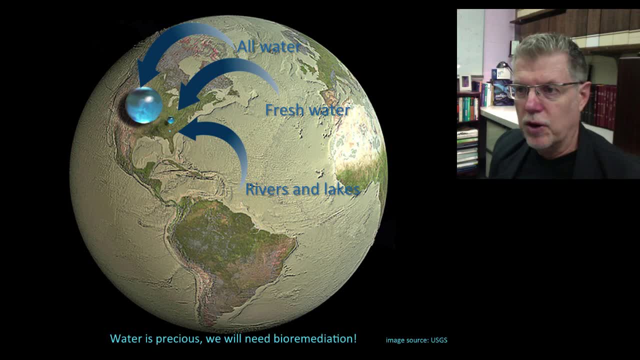 And so I think that bioremediation is going to be a very important tool. It has been in the past, and I think it's going to be even more important in the future to keep our water clean, not only for ourselves, but for future generations. 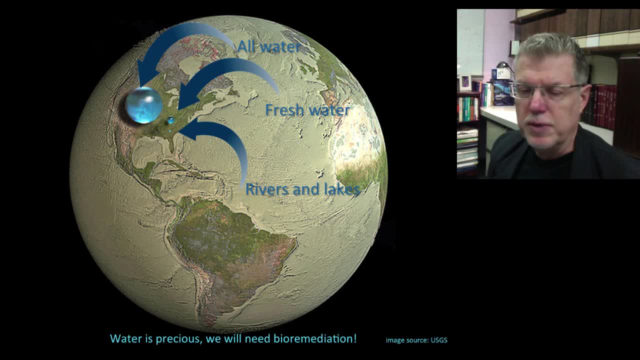 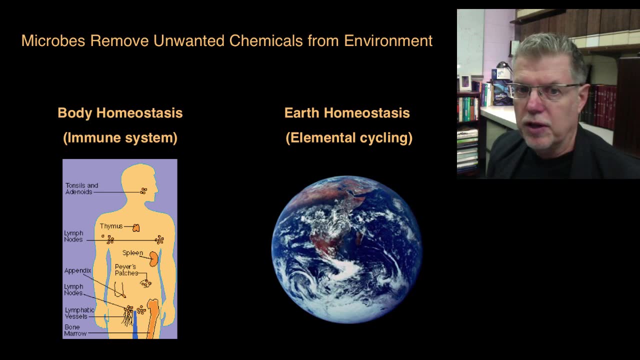 And just to leave you with a last thought about bioremediation is that I like to think about microbes as our best friends in this regard- that by removing unwanted chemicals from the environment- and I'd like to make the analogy here to the human immune system- 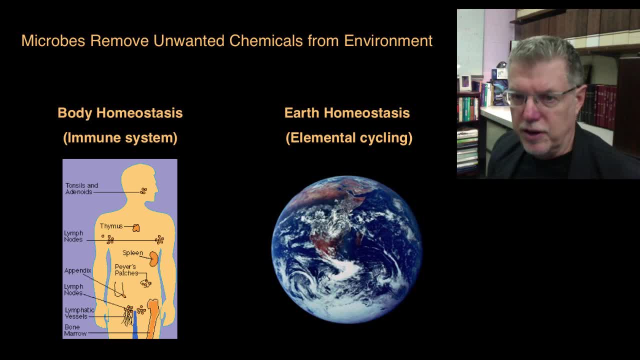 So many of you know that in our bodies we produce immunoglobulins that circulate in our bloodstream and protect us. So by going around and binding to antigens and recognizing foreign things that come into our body, they can protect us from viruses and pathogenic organisms. 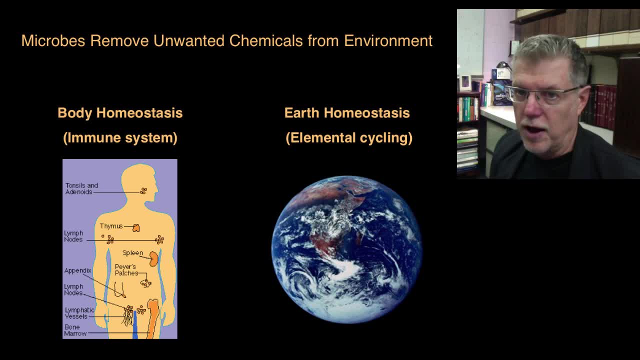 And this is very important to our health. And I think just the same way, if you think on a global ecosystem scale, that bacteria are everywhere. as I've indicated, they're huge numbers, So they're in all of these niches and they've acquired the ability. 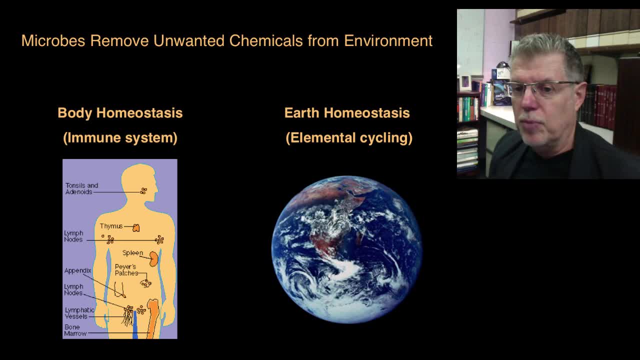 to degrade not only natural chemicals but many of the synthetic chemicals that humans have devised, And so, in the process of doing this, they help keep our planet clean. So if we have spills, we have discharges of chemicals. bacteria are doing their normal thing.